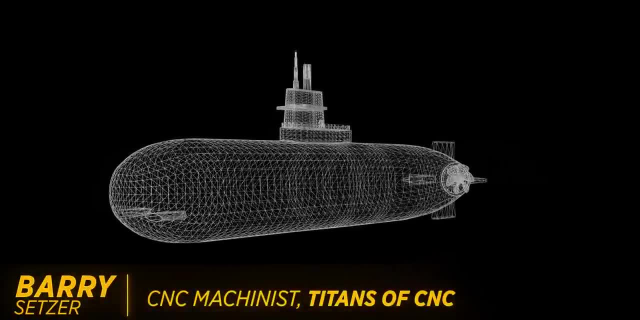 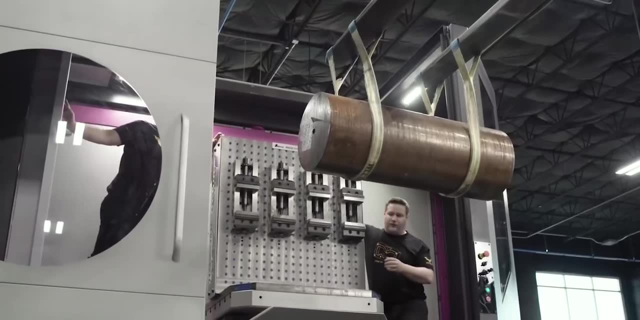 A couple of years ago, my team and I were tasked with machining one of the most critical assemblies of the new Columbia-class submarine. Now I'm not talking about a couple thousand dollar chunk of billet. I'm talking about a 14-foot diameter, 12 million dollar Monell forging with a finished 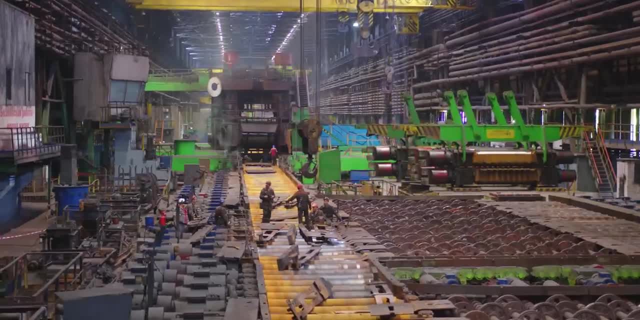 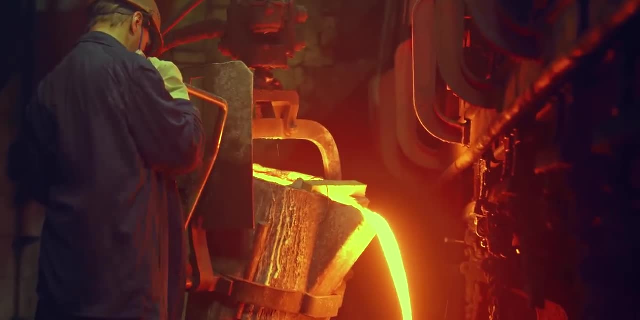 part price of around 50 million dollars. With a piece of raw material like that, you can't just have a little oops and buy another piece of stock. There was only one foundry on earth that we could buy it from, and the lead time was a little over two years. The finished price of this one- 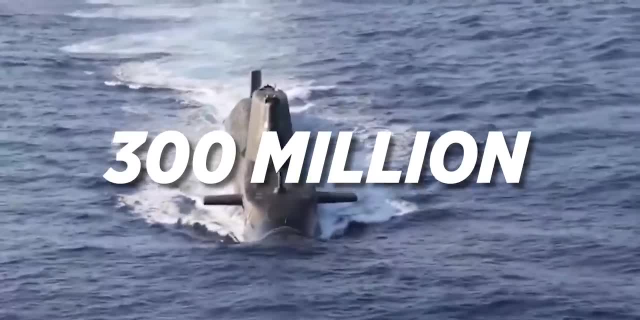 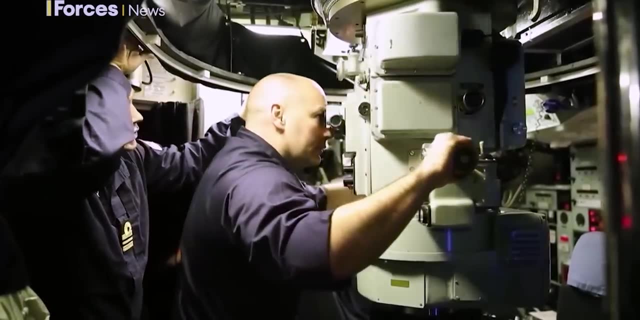 assembly was right around 300 million dollars and our team was making all the parts. This meant that if everything didn't fit together perfectly at assembly, they would know who to blame. Think for a second about the most expensive thing that you've ever made or worked on. 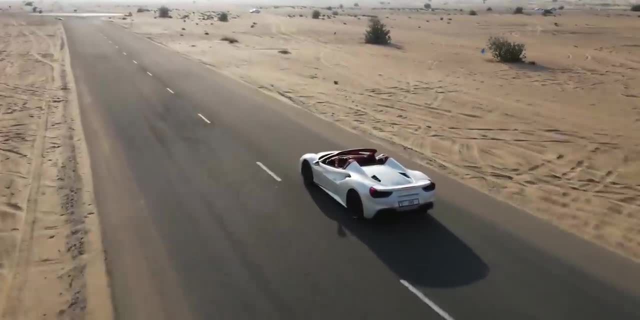 Was it a 900-dollar casting, A 200-thousand-dollar car, A 3-million-dollar boat? How did you feel while you were working on it? Were you worried about making a mistake and ruining your life? Were you worried about making a mistake and ruining your life? Were you worried? 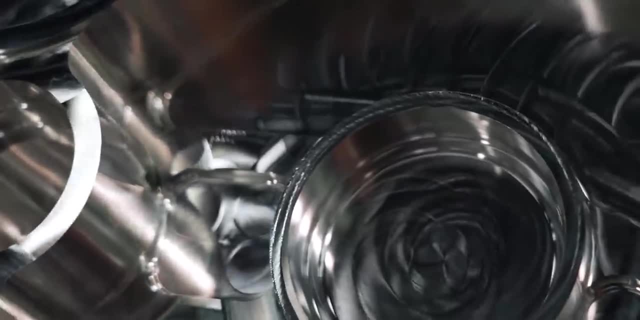 about making a mistake and ruining your life? Were you worried about making a mistake and ruining the finished product? If so, that was a healthy fear. It's always kind of nerve-wracking when you're working on something expensive. One mistake can turn a ten-thousand-dollar chunk of material. 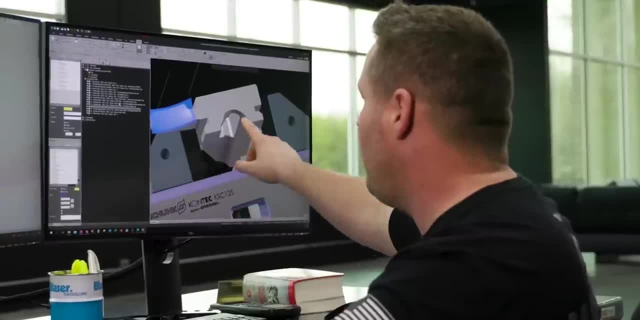 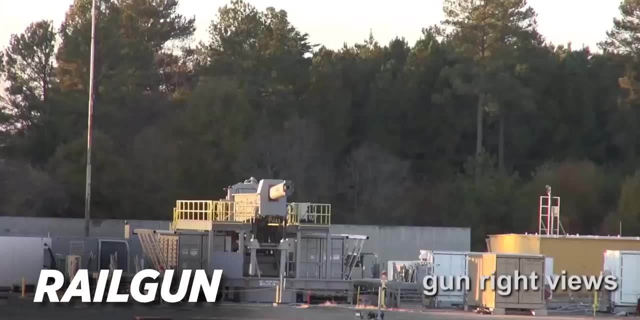 into workless garbage. Now, me and my team were no strangers to making insane parts for some awesome applications. We'd work together on projects including the electromagnetic railgun which fires a projectile at Mach 7, hypersonic glide-body missiles that fly over Mach 17,. 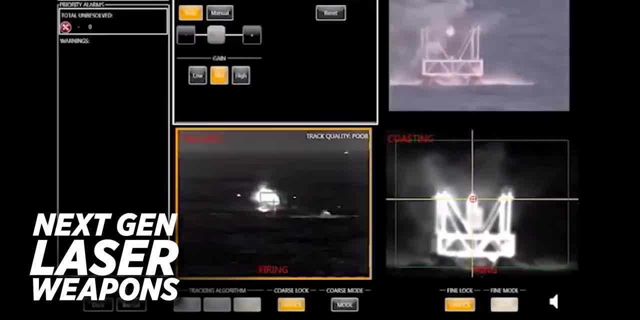 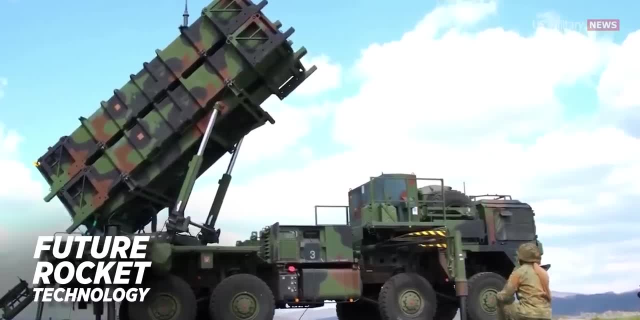 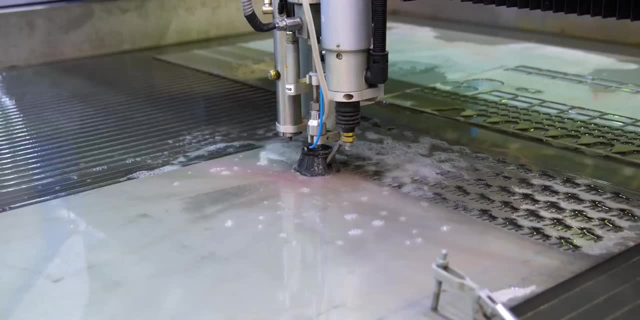 next-generation laser weapons mounted to ships and saddles, satellites, nuclear reactors for space, next-generation fighters, drones like the Reaper and Predator, future rocket tech- you name it. After a while, you don't even blink when someone throws a ten-thousand-dollar piece of white sapphire on your desk and asks you to water jet. 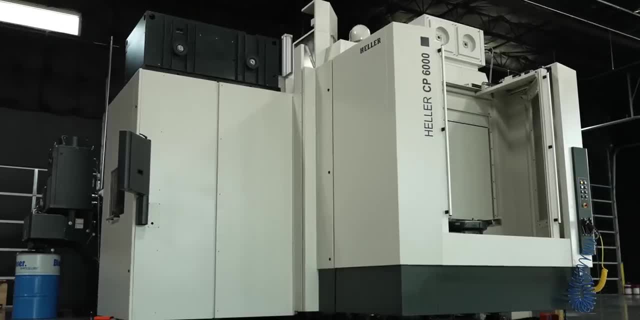 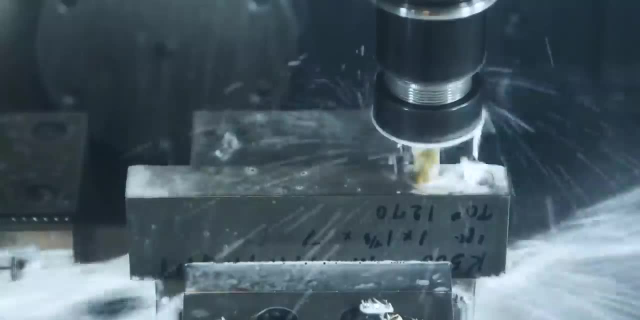 it Just another day, But with a price tag in the hundreds of millions of dollars and zero margin for error, this particular job made us a little nervous. Monell wasn't a material that we ran a lot of, and this group of parts was going to take us several months to machine. We did a lot of research and 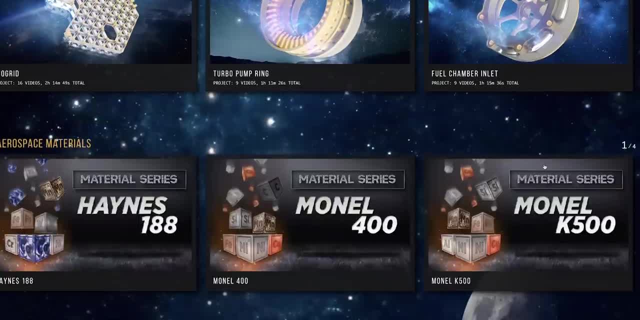 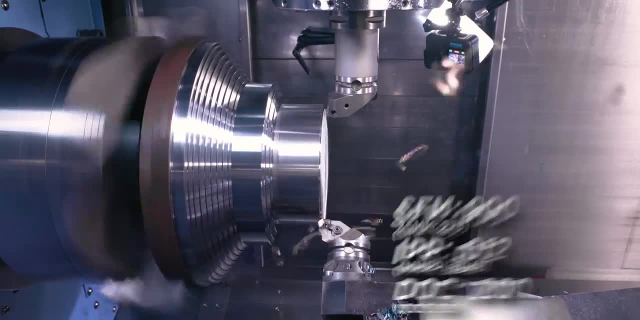 including visiting the Titans of CNC Aerospace Academy and videos that Titan himself had done on machining Monell. This was also the first time that we decided to use Kenna Metal inserts at this company, because Titan and others swore by them for tool life in these materials And those inserts are. 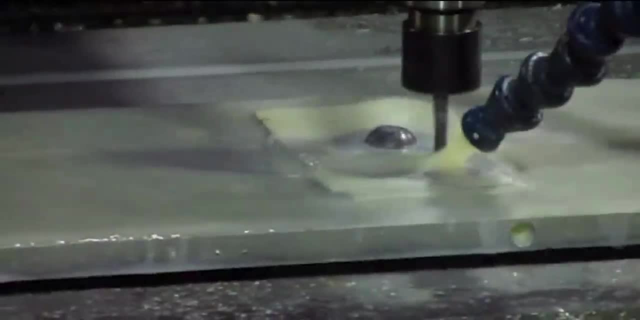 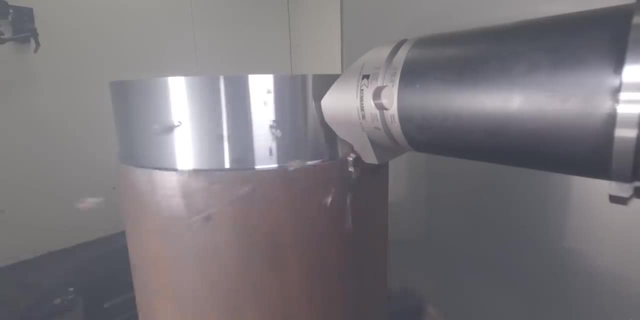 still being used on that job to this day. You might be making aluminum washers and a beast part like this may not seem relevant to you today, but tomorrow, who knows what you're going to be making? As you gain an experience and reputation, the parts you make are going to get more complex. 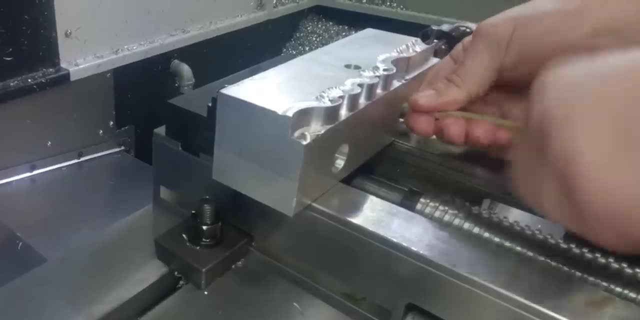 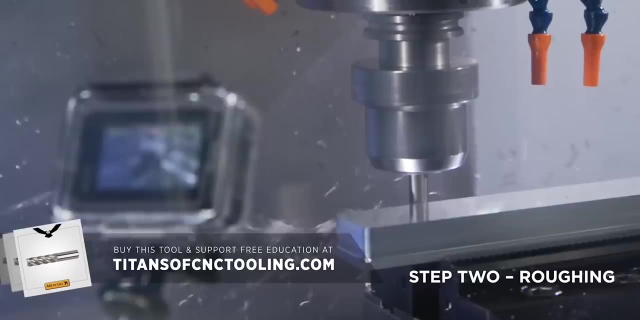 every day. You have to hone yourselves and your skills on the small stuff so that you're ready when you get to the big stuff. Nobody starts their career making million-dollar parts, and there's a reason for that. Everyone is scrapped apart, and it's way better to learn some of these lessons on. 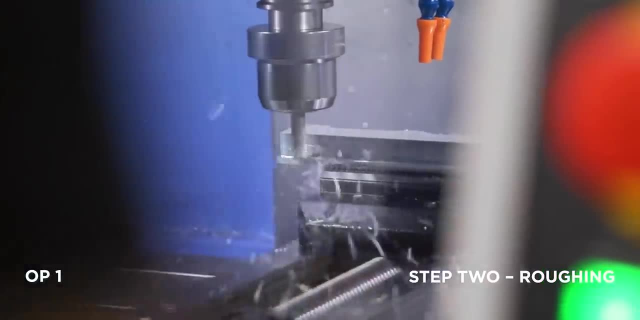 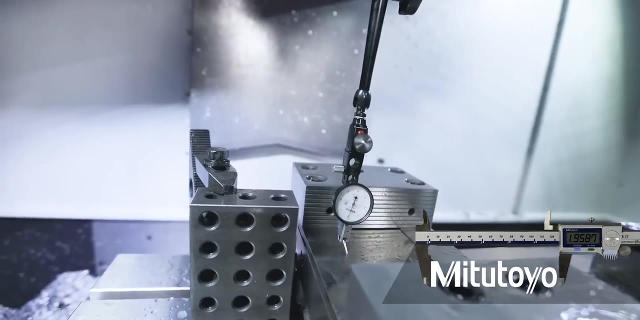 a two-dollar chunk of aluminum. The beginning of your career is where you build the foundation for what you'll eventually become. Start with good habits: keeping everything spotless and organized. ask for help when you need it, stay open-minded, collaborate with your team, learn from every. 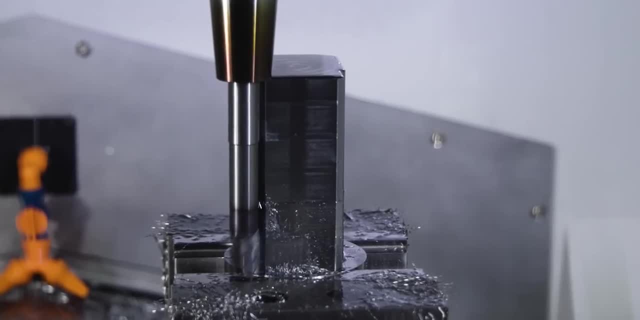 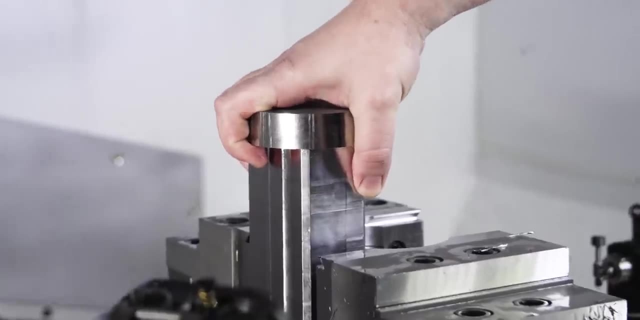 previous job and all the way to the top. That's what Monell is all about. He's going to teach you how to do it. Always build on your personal skill set. Once everybody knows that you can be trusted to make a $20 one-off part without fail, they'll start trusting you to make the $200 parts and before. 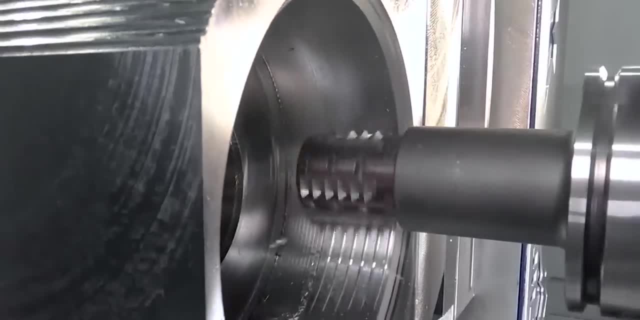 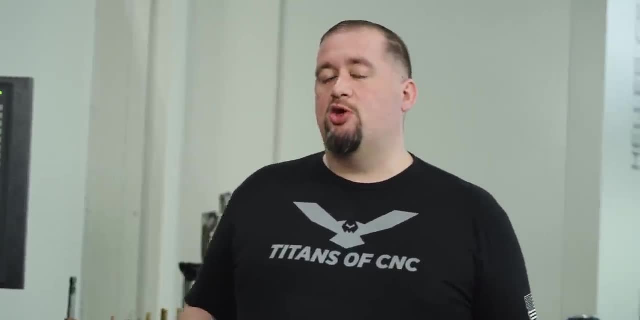 you know it, $200,000 seems cheap. So how do you even approach a $50 million part or a $300 million assembly? Now, before we get into that, if you guys appreciate what we're doing and you want to help us support free education, you can click the join button and become a member Now by becoming a 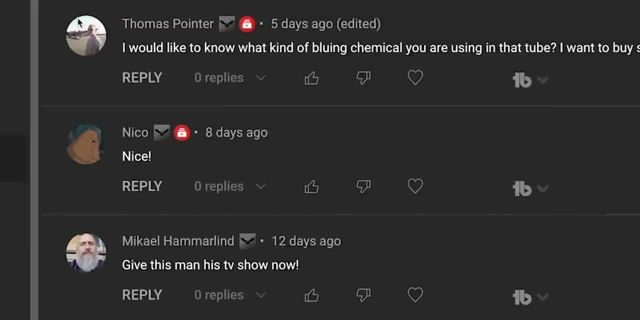 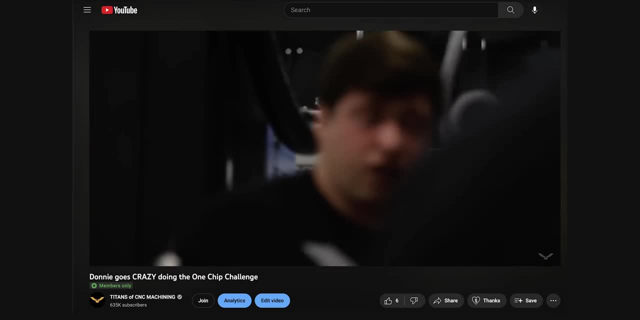 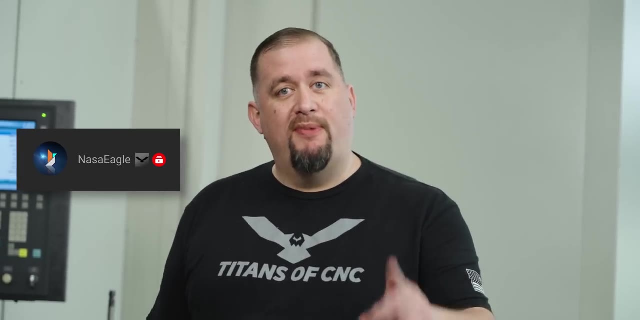 member. you're going to get some awesome perks, like you're going to get badges by your name, you're going to get access to our Discord server to chat with me and the team, and you're going to get exclusive content and free merch And shout out to NASA Eagle for becoming one of our first members. 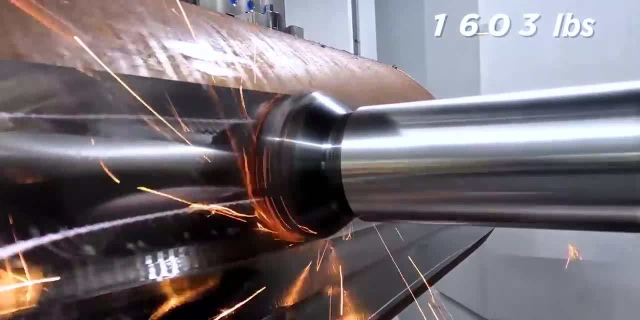 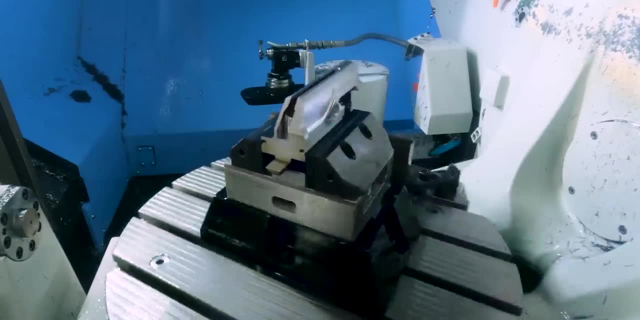 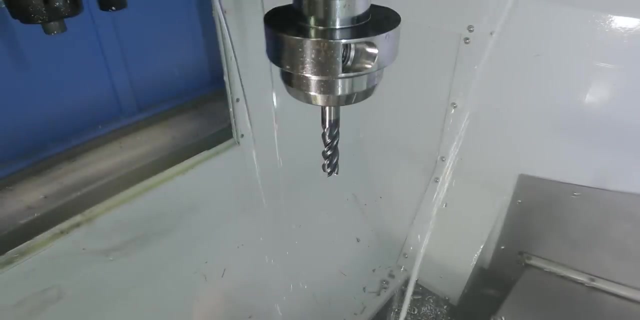 Well, we started by gathering together a group consisting of our most experienced programmers, machinists and manufacturing engineers. Together we discussed everything from fixturing the cutting tools- ambient temperature of the shop- to the machines we would use the properties of the material tool, life, you name it. We discussed every single step of the